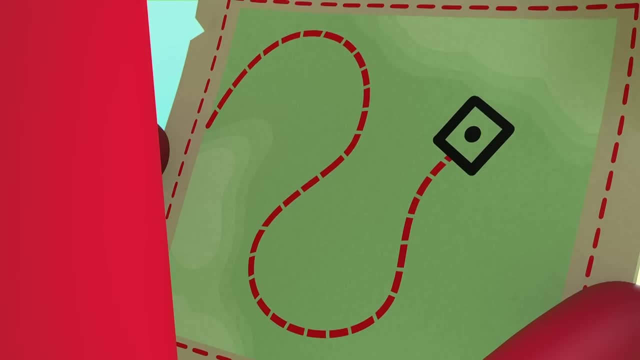 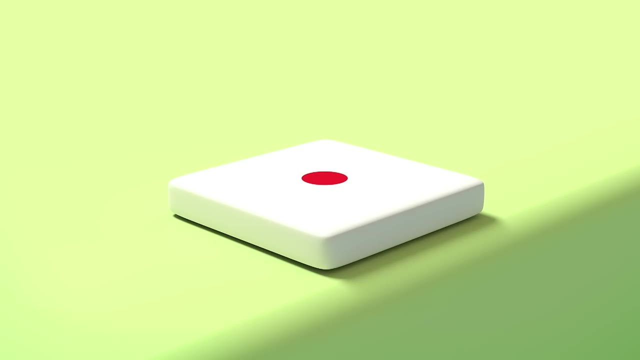 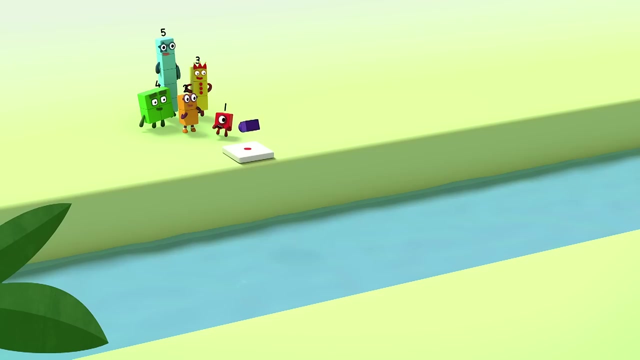 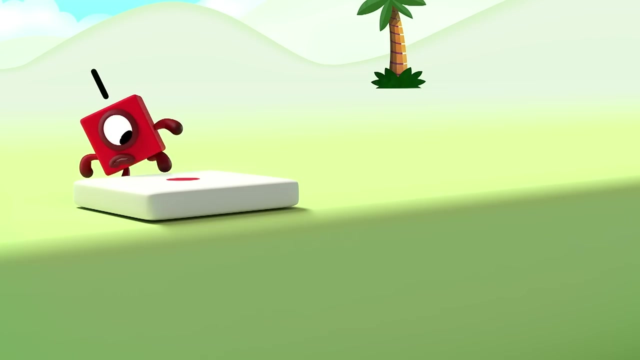 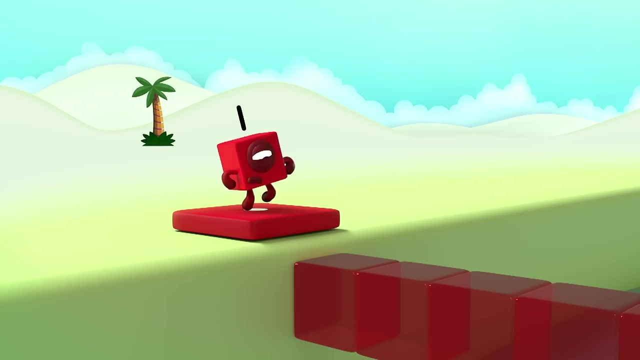 If the map is right, the Pattern Palace should be right here. Welcome to the Pattern Palace, where you can play all day, But first you must cross the Pattern Paths. Be brave and step this way. Follow the Pattern. Here I come. 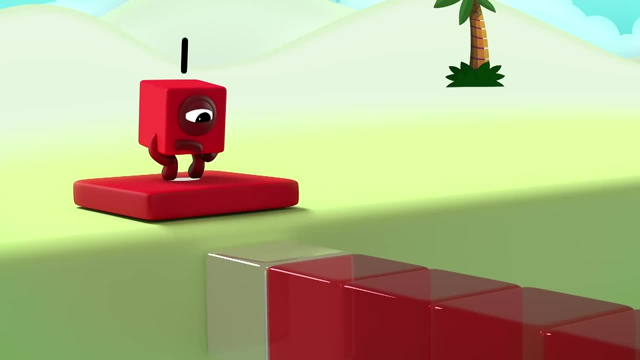 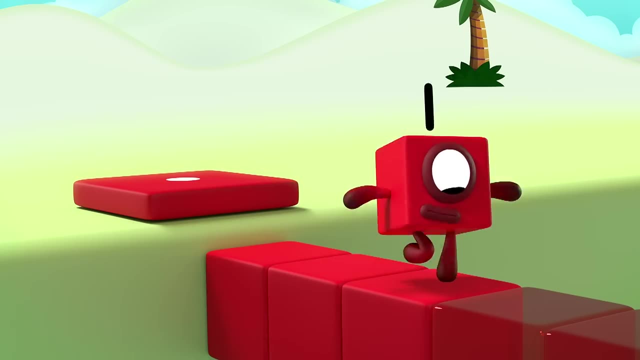 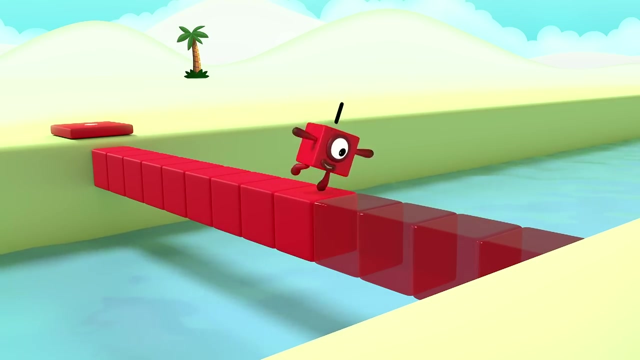 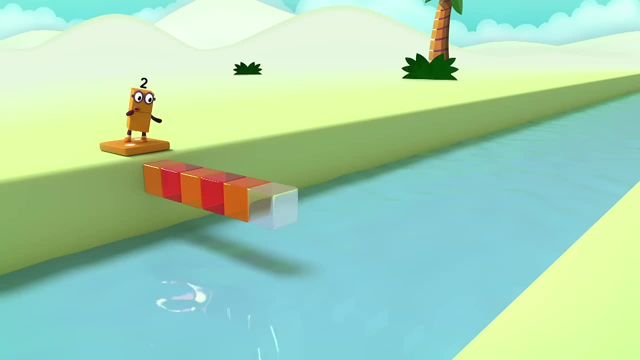 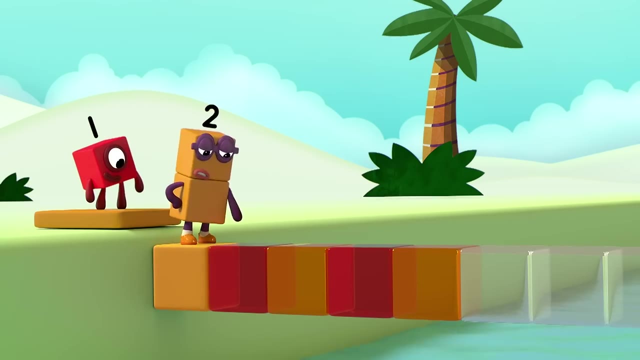 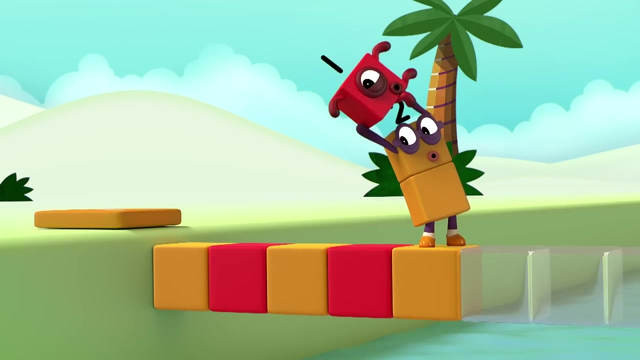 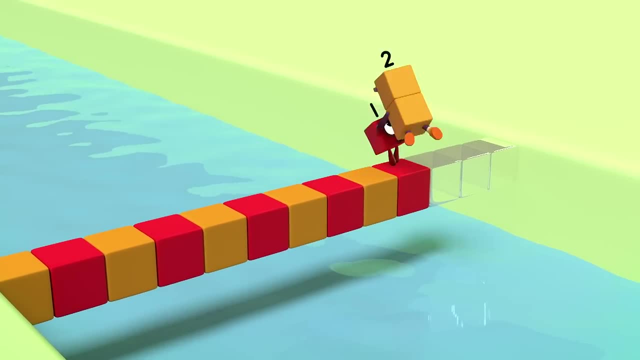 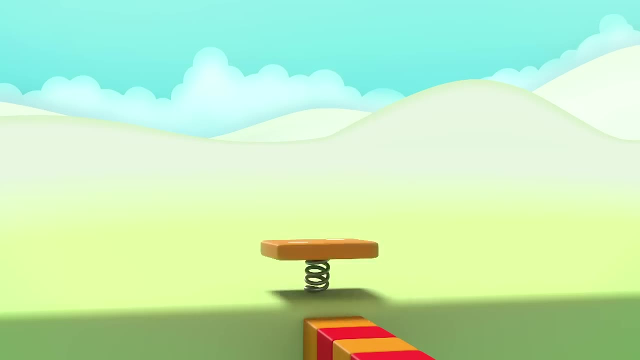 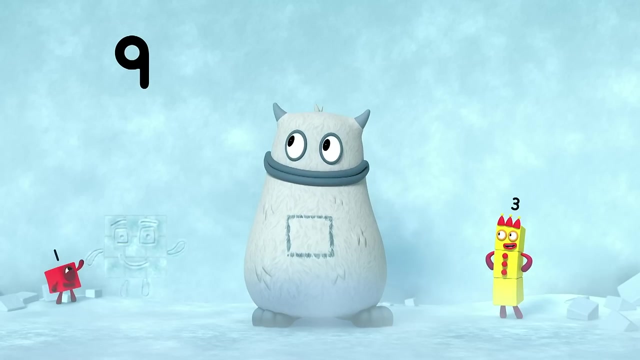 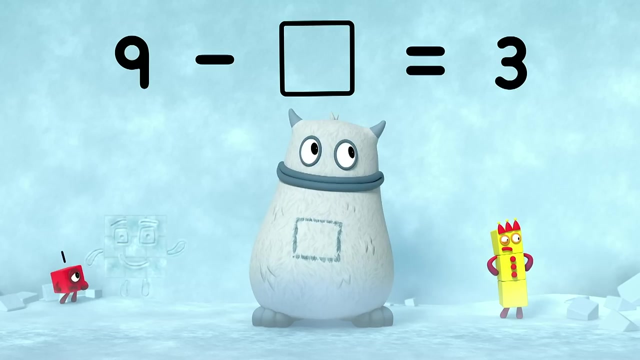 Orange, Red, Orange Pattern unlocked. You can count on us. we're the number blocks. Nine minus Young equals three. So what's missing? Hmm, Come over here. three. Hey, Brr, That's one. 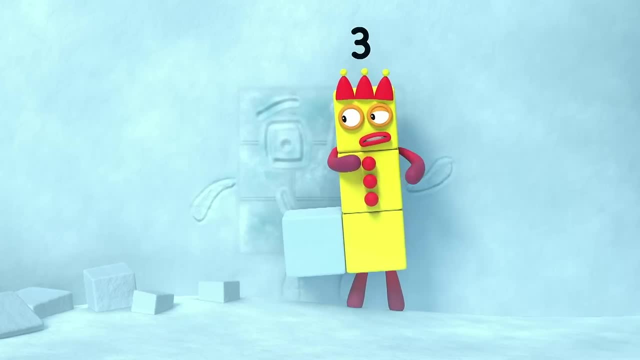 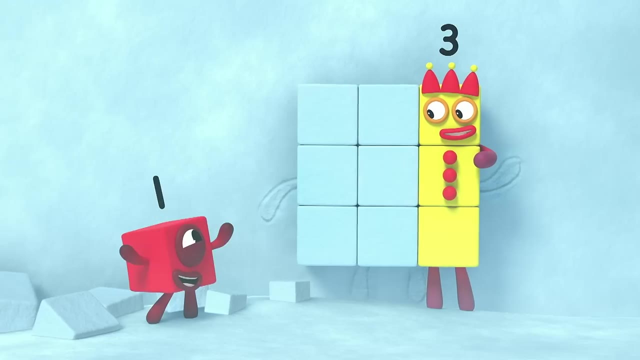 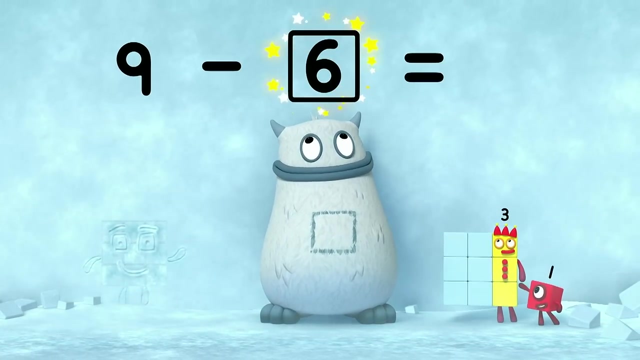 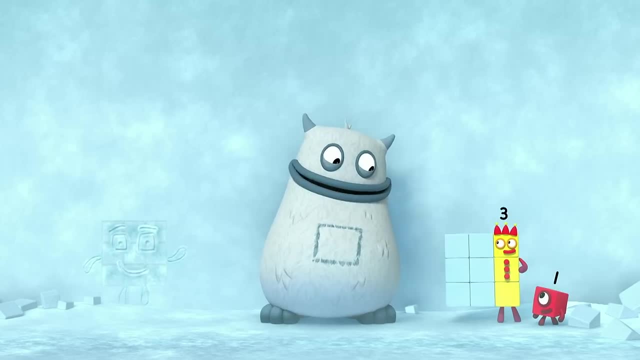 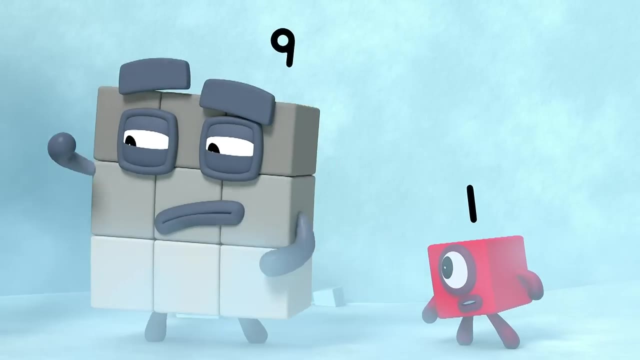 Three And six is in your tub. Yum yum. Well done. Oh Whee Woo, It's good to be back. Where are the others? Oct Cell Block turned off. Yum, Yum, Yum. 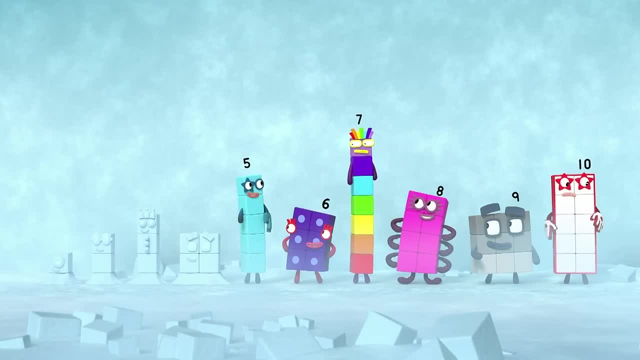 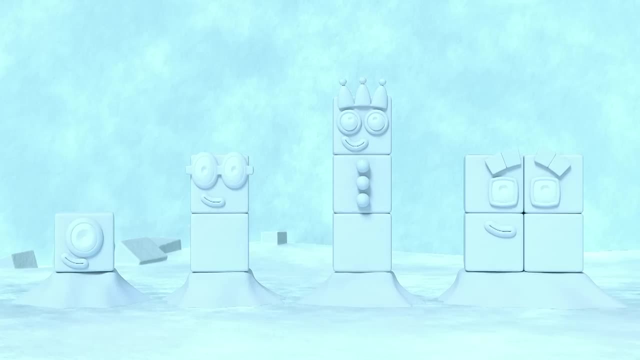 Yum, Everybody. stay close. no need to panic. Uh, What's wrong, friends? Why don't you? Oh, they're made of snow, S-s-snow, yeah, Yum, Oh, Yum. Who's in my tum? 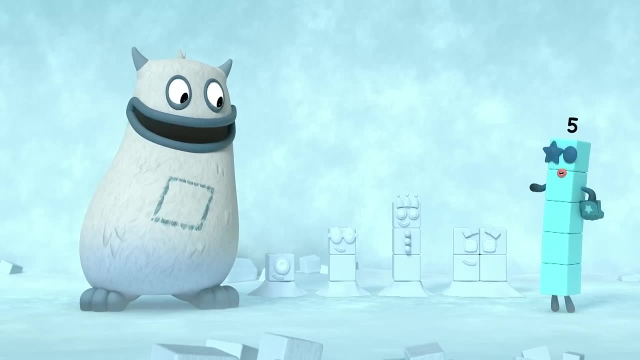 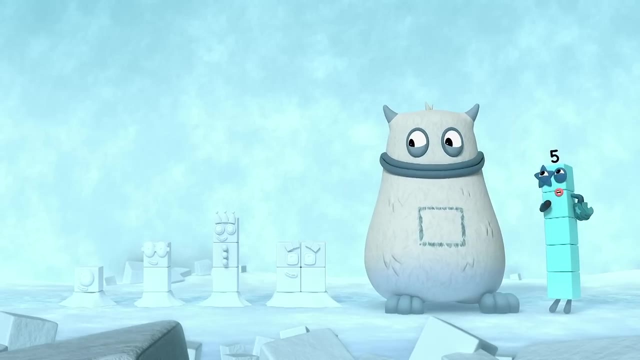 That's easy. The real one, two, three and four. Nope, They're all together now. So what do they make when they're all together? One plus two plus three plus four equals Yum. Let's try adding the snow blocks together. 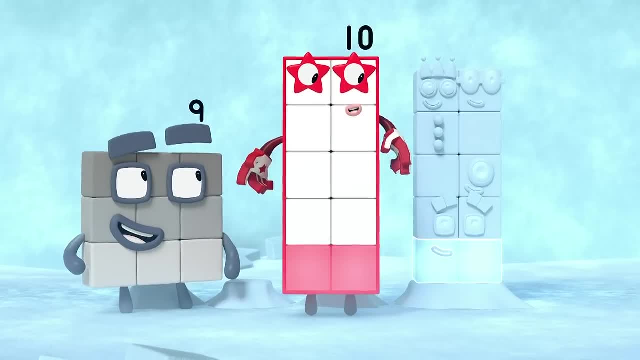 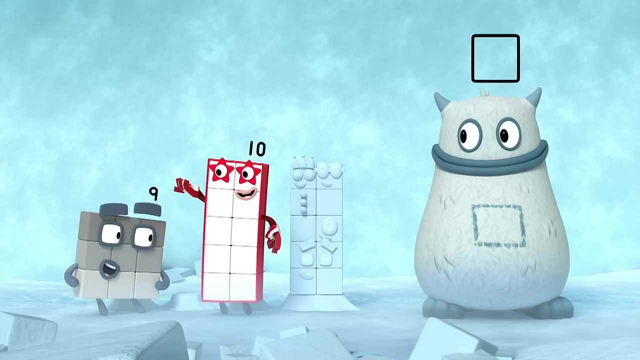 One, two, three, four. One, two, three, four, five, six, seven, eight, nine, ten Ten snow blocks. So one plus two plus three plus four equals ten. There's a ten in your tum. 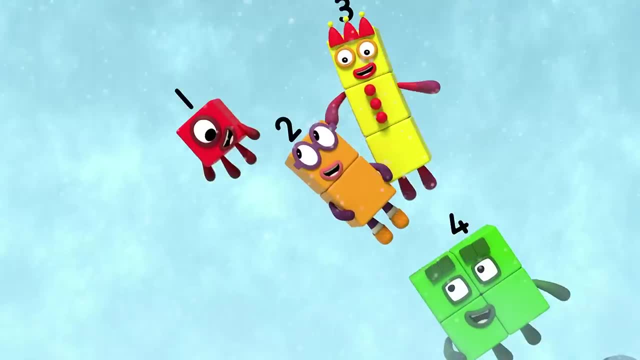 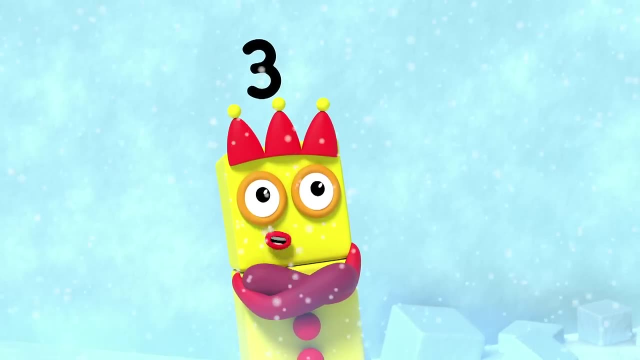 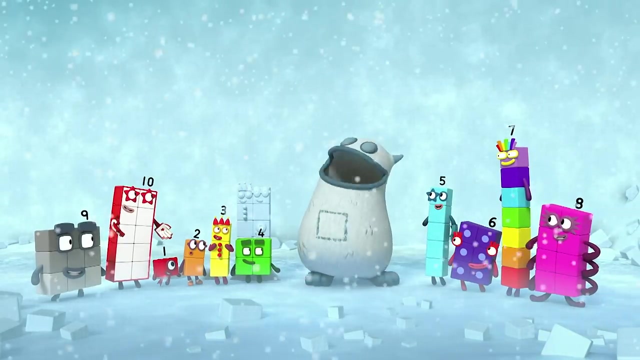 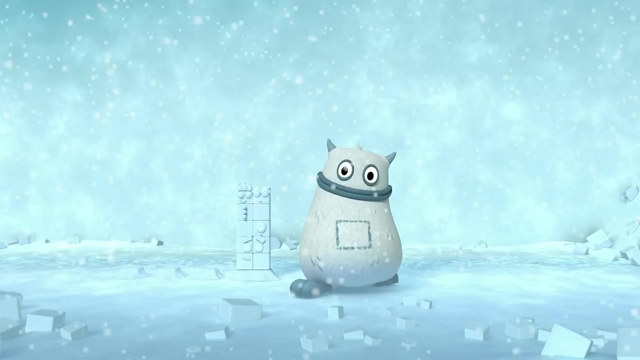 Yum, yum. Well done. It's nippy out Much warmer inside. Can we all come in until it stops snowing, please? No problem, And plenty of room for you too. You can count on us. we're the number blocks. 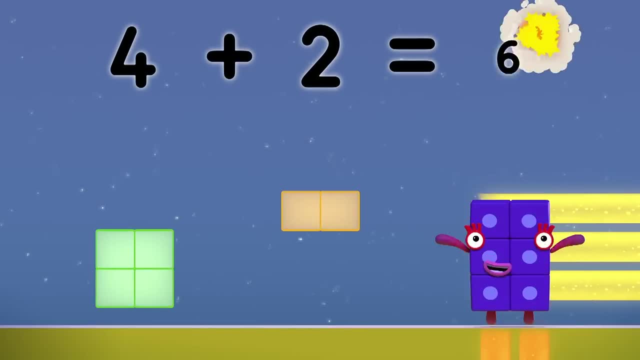 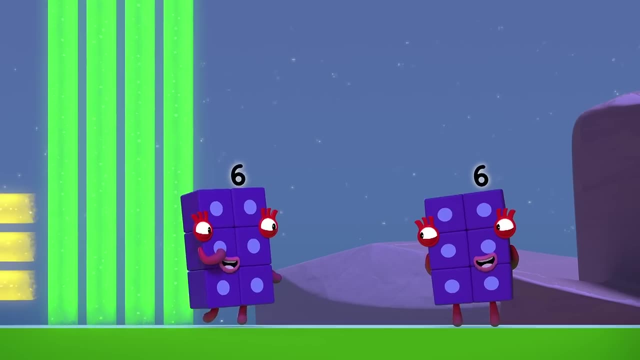 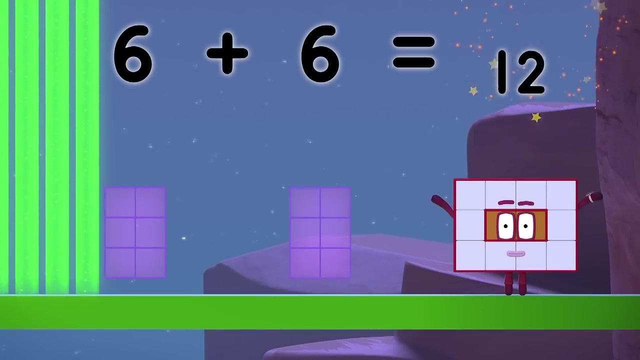 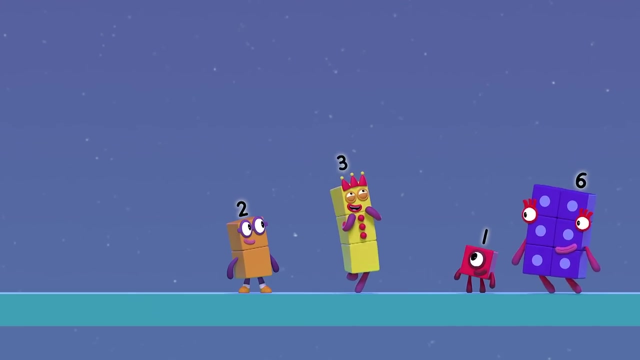 Four plus two equals six. I'm so glad I can reach this shelf, So happy I'm beside myself. Six plus six equals Twelve. Oh, well done. Who came up with this idea? Me, me, me. Three plus two equals. 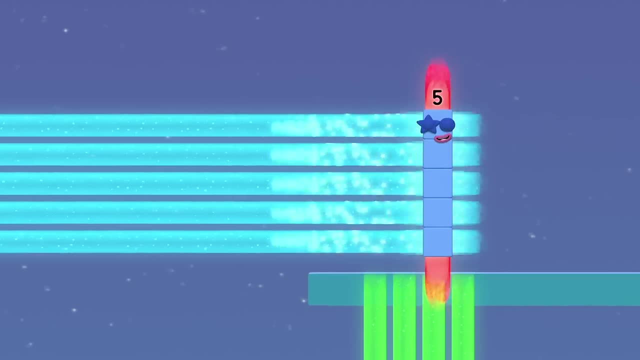 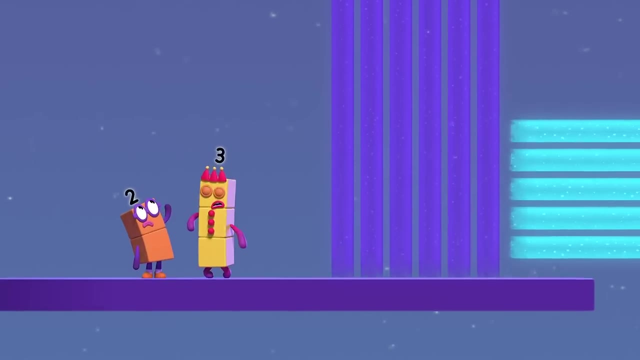 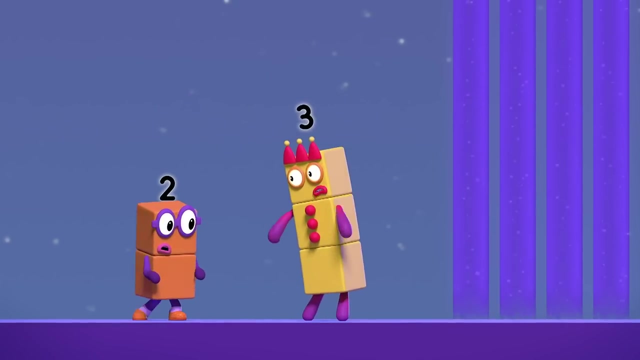 Five Hooray, Yeah, Um, but how do we get up there? We can't do that. We can't do that. We can't make anything. that's six blocks wide. We've only got five blocks between us. Hello, my friends. 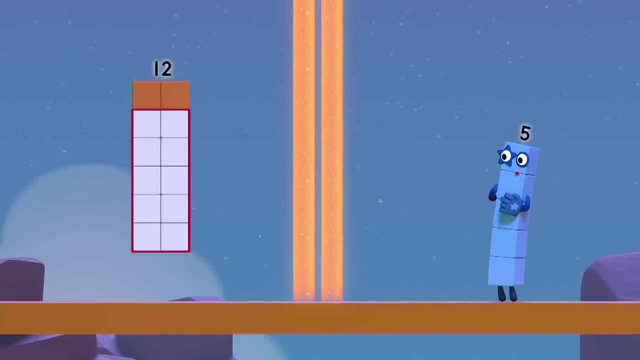 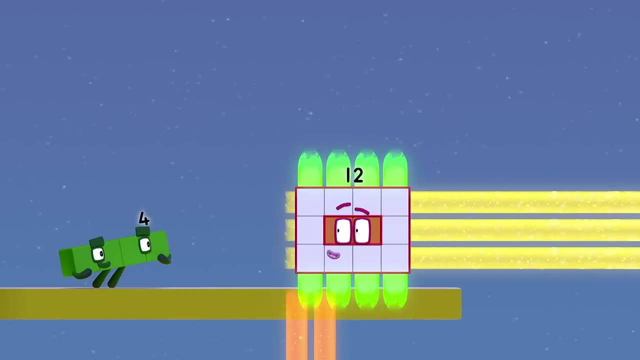 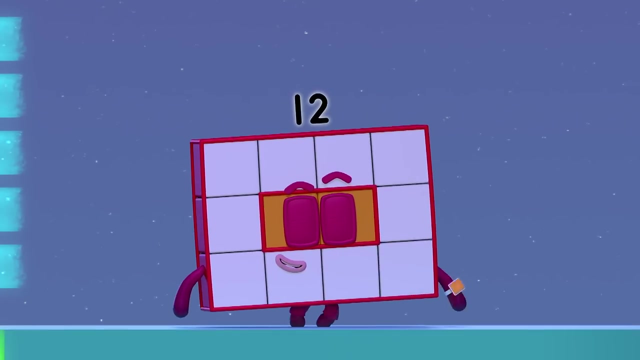 Twelve Switch. Congratulations on getting so far, Switch. By working together, you've nearly reached the top. What a super rectangle. But not even I can make every size of rectangle. I can't make a rectangle that's five blocks tall. 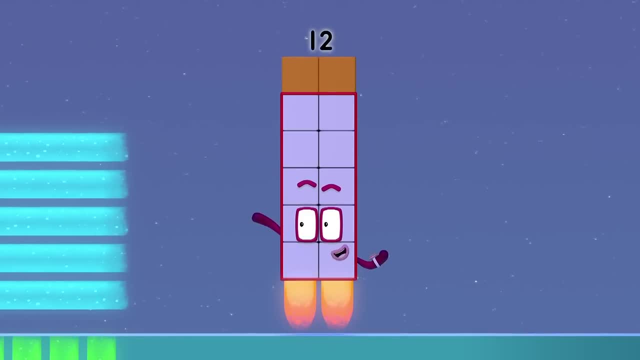 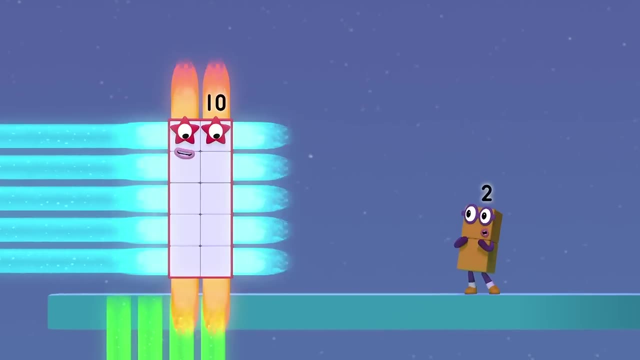 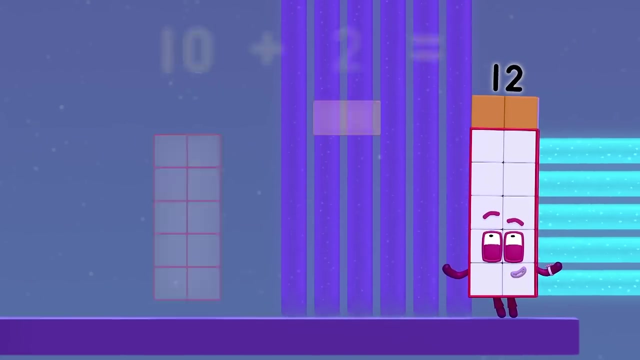 See, But like you said, Three. Sometimes there's more than one way to solve a problem. Twelve is ten plus two. Ten plus two equals Twelve Ten. I'll drop you a line: One, two, one, two. 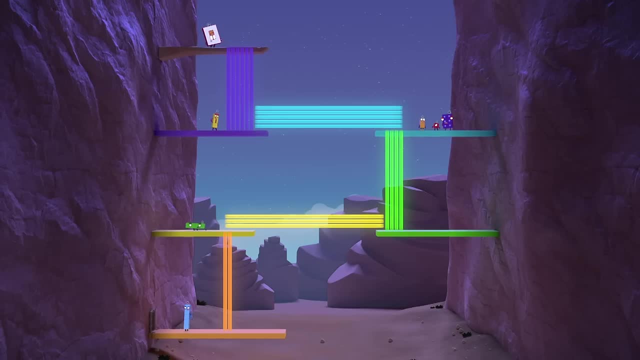 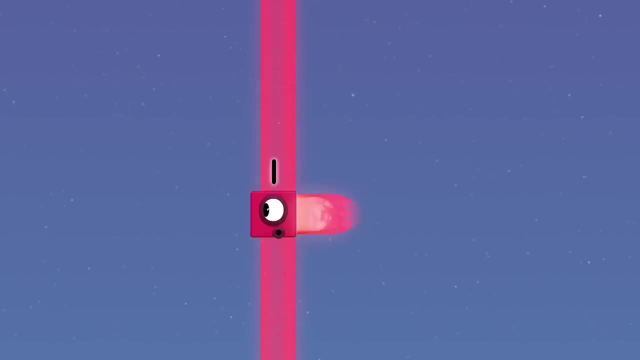 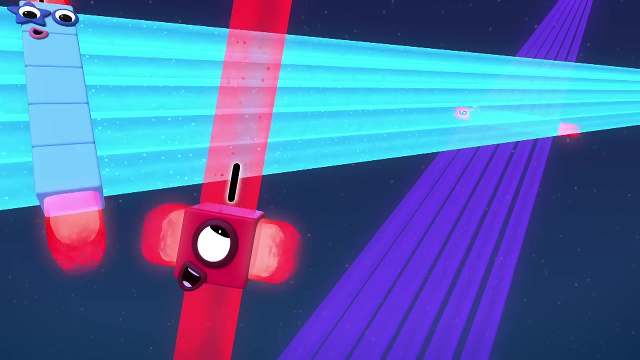 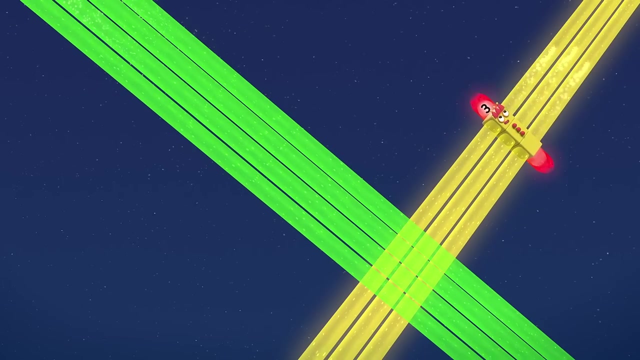 Half Ten plus two is 55. And that's ridden it over. Whoa Strike Opp. Oh man. A U U R A, Ooh a. I think I know what this looks like. 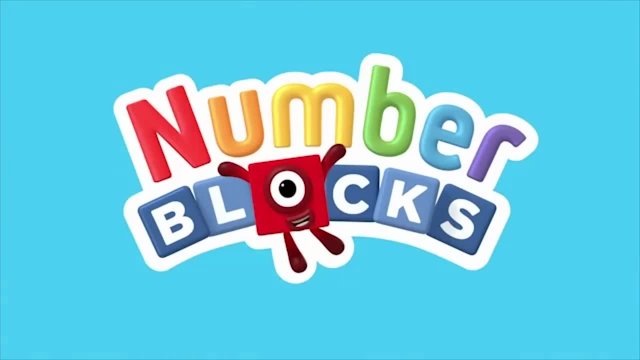 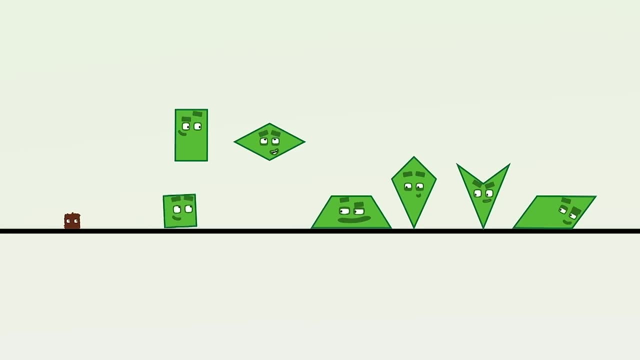 Oh yeah, Four-sided shapes, introduce yourselves. Rectangle Rambus, Trapezium, Kite, Dart, Parallelogram, Square. Ooh, what wonderful names And what wonderful shapes. Rectangle Rambus. 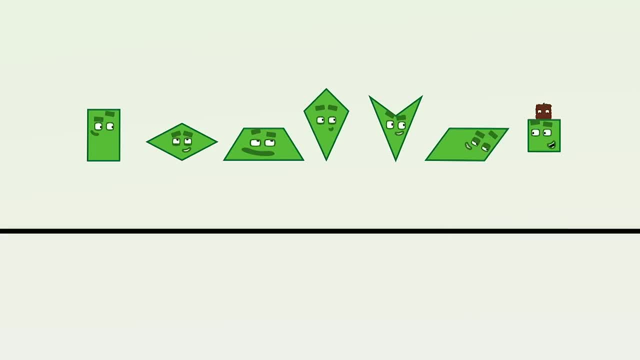 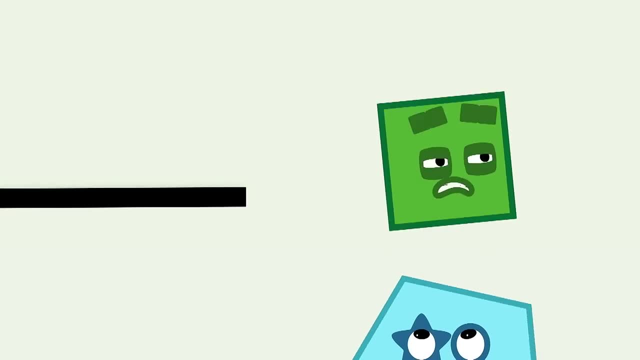 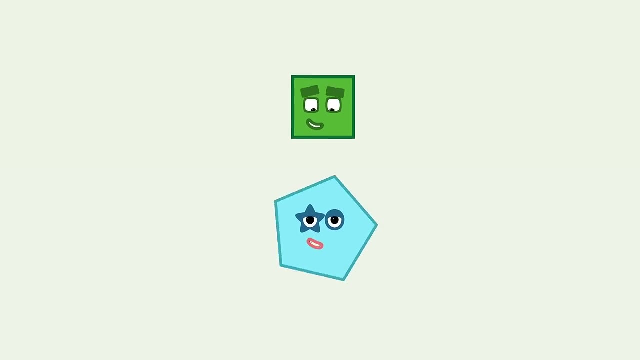 Trapezium, Kite Dart, Parallelogram Square. Ooh Squarey, come back. Oh hello. Who are you? I'm a pentagon with five sides, High five. Let's have a hexagon in the mix. Count my sides and you'll find six. 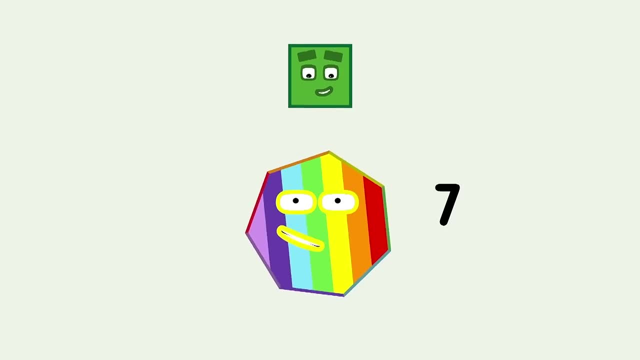 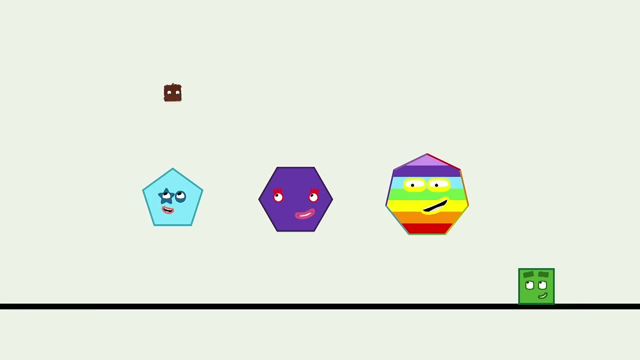 And, lucky me, I've got seven sides. I'm a heptagon, A heptagon, Ooh. One, two, three, four, five sides pentagon, Six sides hexagon, Seven sides heptagon. 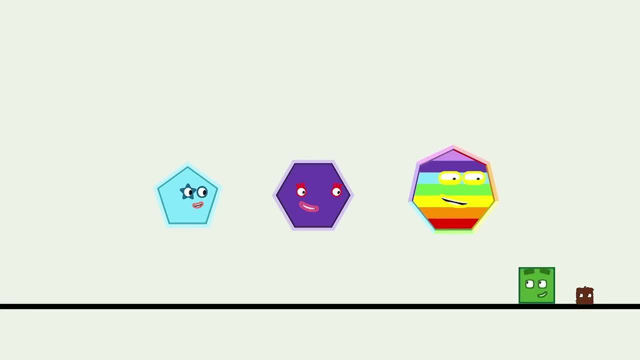 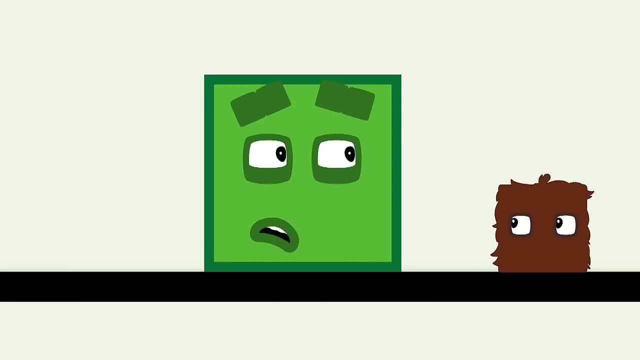 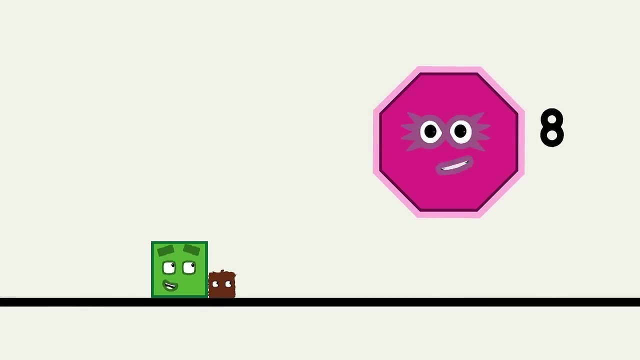 Ooh, what wonderful names And what wonderful shapes. What's that, Squarey, You're ready to go home? Hey, Have no fear, Octagon is here. One, two, three, four, five, six, seven, eight, Eight sides. 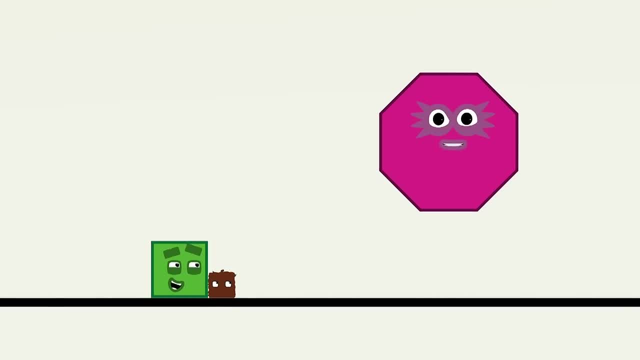 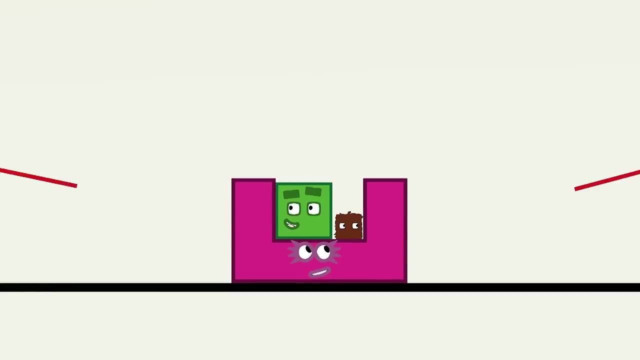 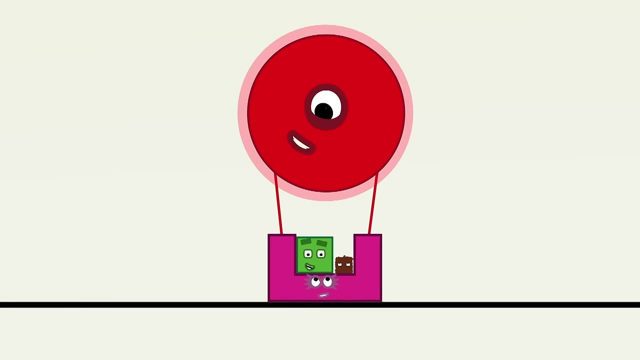 I will get you home, Octagon, Make an eight-sided flying basket. One, two, three, four, five, six, seven, eight Basket. I'm a circle. I have just one curved edge. Hold tight, folks, Here we go. 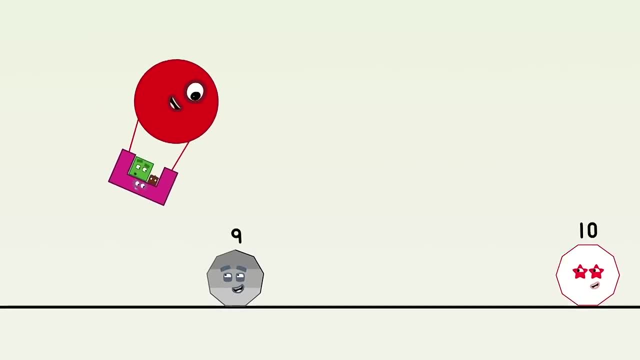 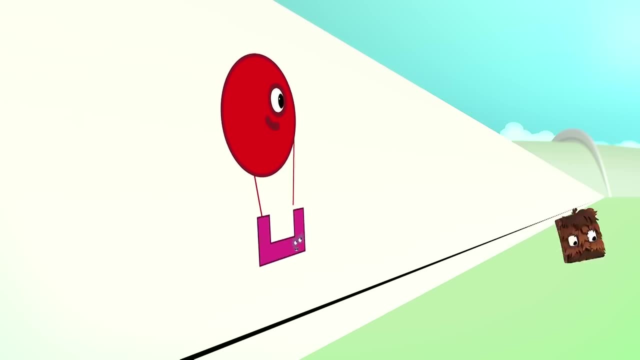 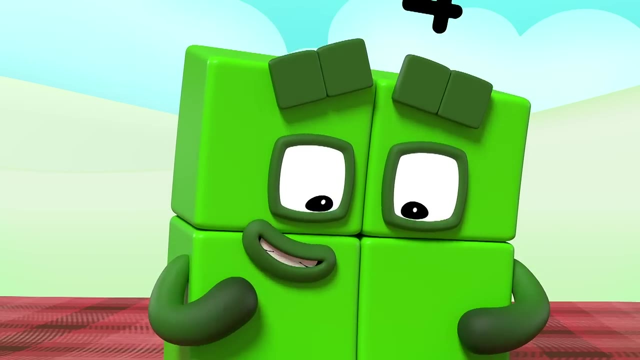 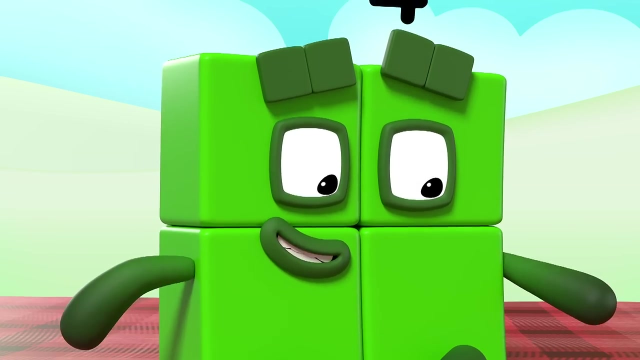 Hooray, Ooh, Wow, Good-bye new friends. Ah, I'm me again And you're you. We went to Flatland and Triangles were there and a rectangle and a pentagon and I was a real square. 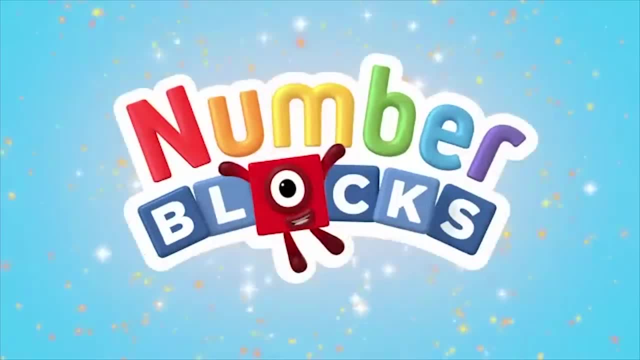 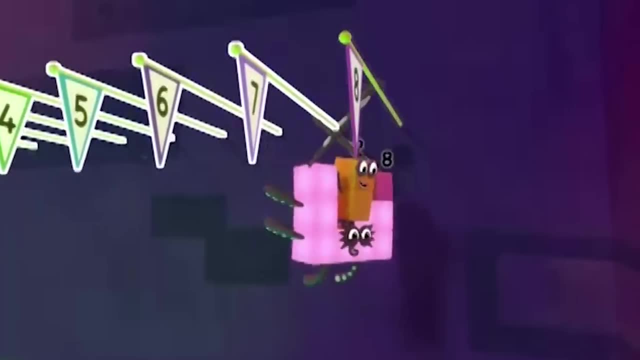 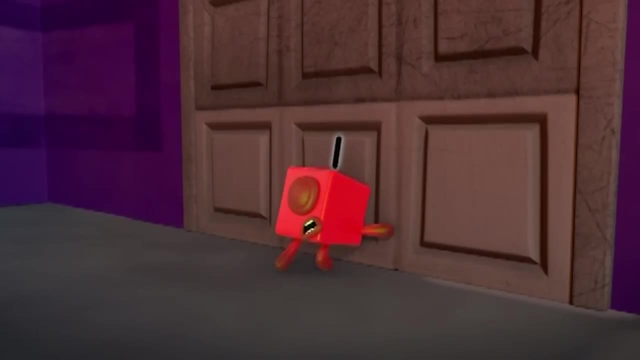 Yeah, Hooray, Hooray, Hooray Ha. 1,, 2,, 3,, 4,, 5,, 6,, 7, 8.. Swing, It's stuck. Squares are strong. Let me try. 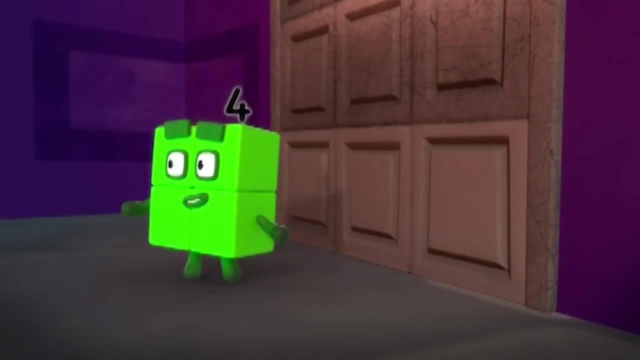 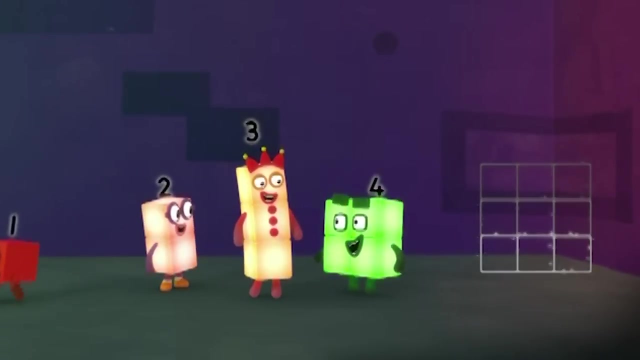 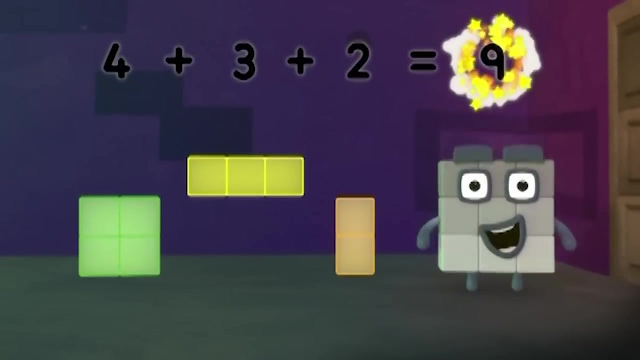 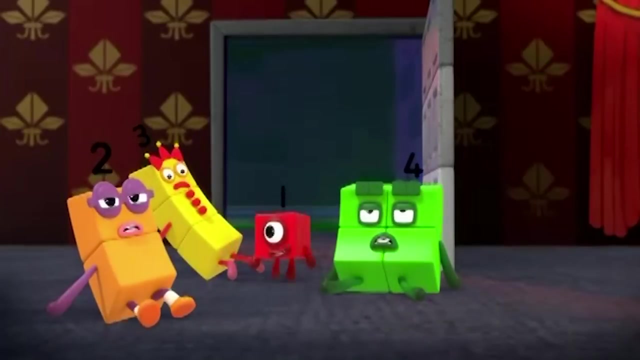 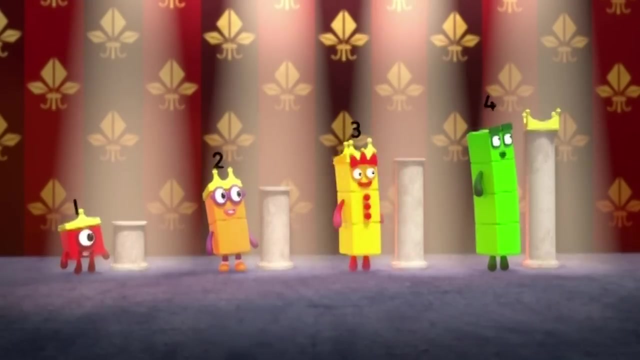 We need a bigger square. 9!. How do we get 9?? 4 plus 3 plus 2 equals 9.. Thanks, 1, 2,, 3, 4.. 4 crowns 2. 2!.